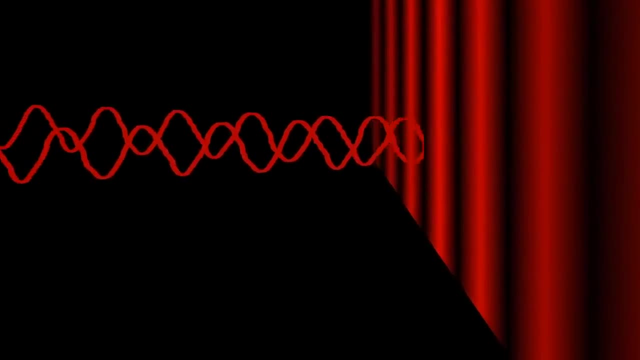 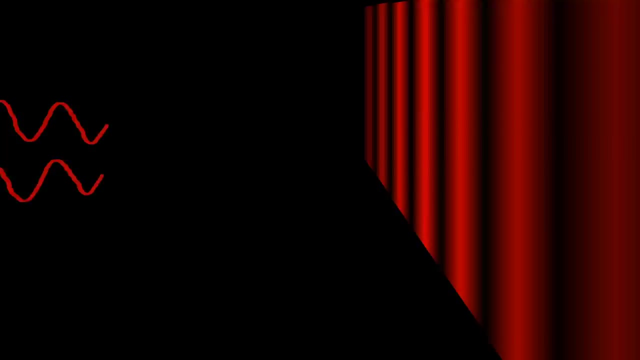 Which means when this light is arriving as a crest, the light from the other slit is arriving as a trough, And so they cancel each other out. But if you go further left you see another bright spot, because now the light from one of the slits has to travel a full extra wavelength. 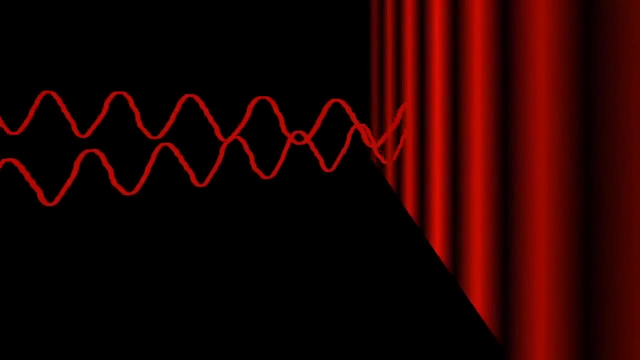 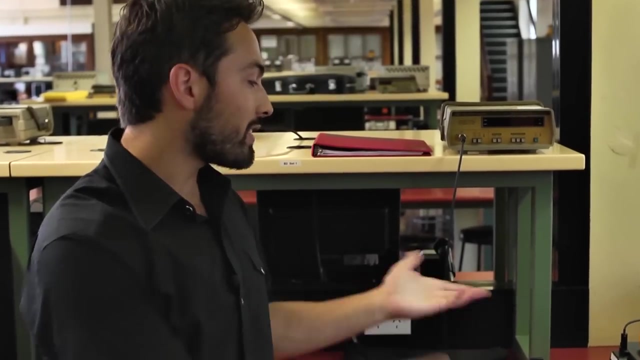 compared to the light from the other slit. and so again they arrive in phase, Crests with crests and troughs with troughs, creating constructive interference, and so we see a bright spot of light, And that's how the whole pattern is created. 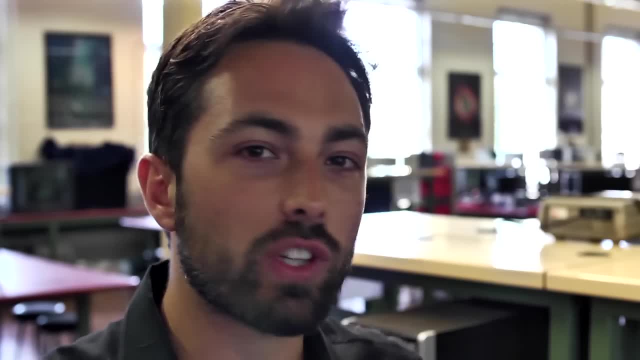 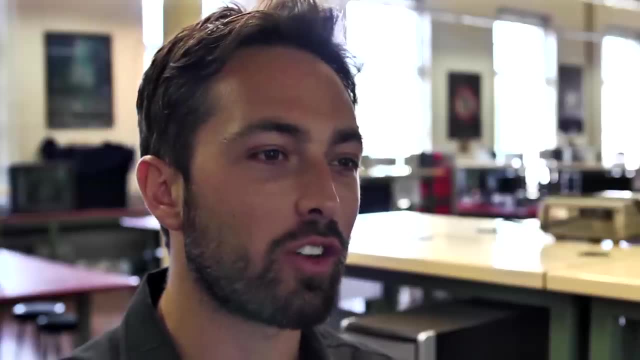 But what if I decrease the intensity so much that there wasn't a whole wave of light going through there, there were only single photons. Then how could they interfere with each other? because there's only one in the device at any one time. So would we still see an interference pattern? 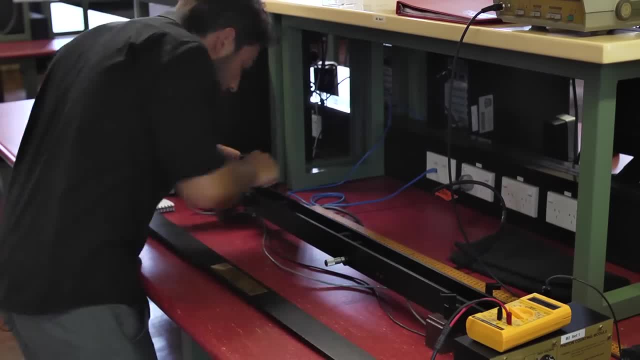 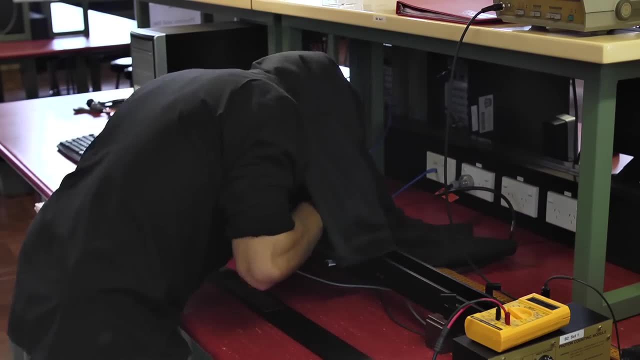 That is what we're going to find out. In order to make this work, I had to line up a very faint source and to see where the light was going I had to shroud my head in that black cloth, But I finally have the apparatus ready. 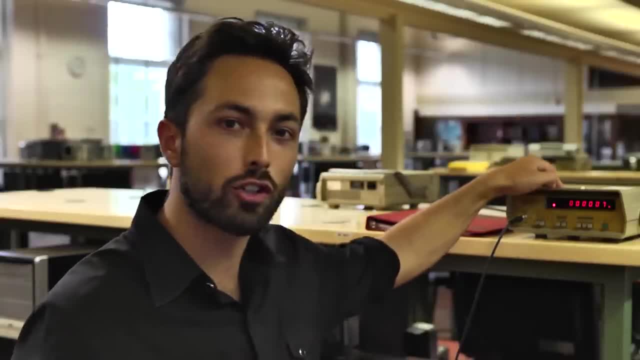 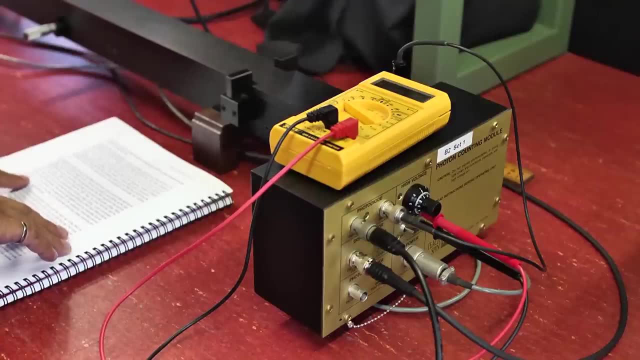 You can see, up here I have a frequency counter which actually counts the number of photons received per second at the detector. The detector is a photomultiplier tube which is capable of detecting single photons. It's like a very sensitive eye, like the frog's eye. 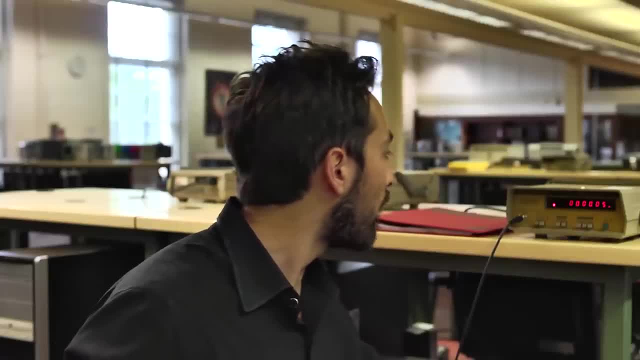 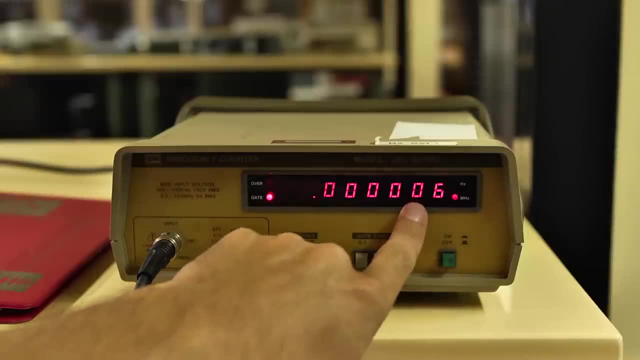 Now, right now, there's no light passing through to the detector, but there is still a bit of a background reading, and that's because I can't block all the light out of there. plus, there are cosmic rays passing through this room, which will also set off the detector. 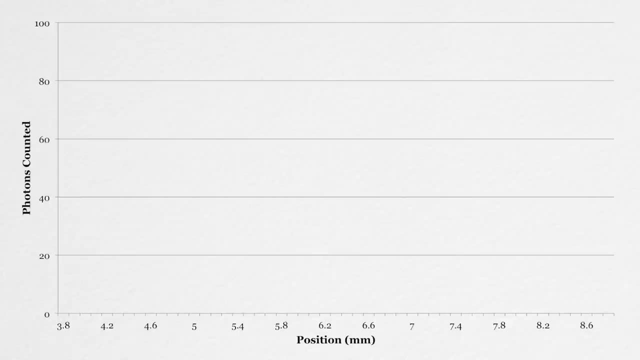 I'm plotting a graph of the number of photons counted as a function of position across the detector. If you have a look after one second, the distribution seems random. There doesn't seem to be any pattern in the arrangement of those photons as they hit the detector. 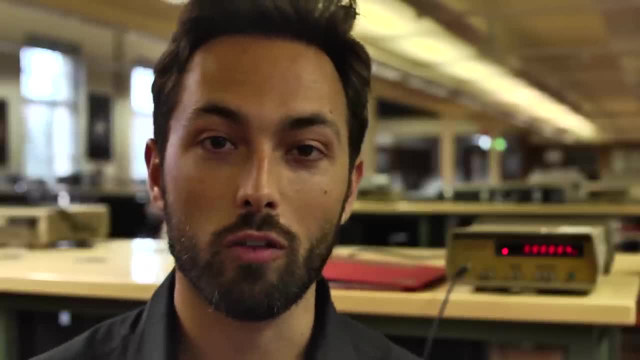 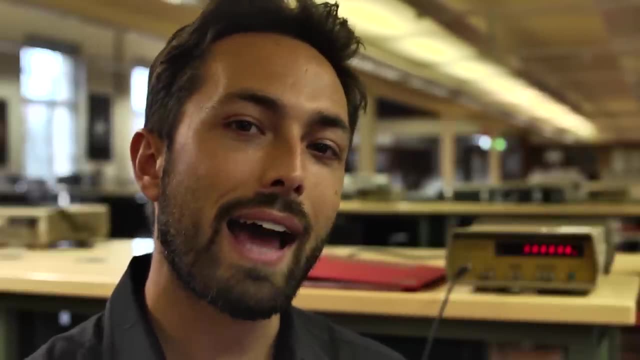 So maybe it's true: a single photon can't interfere with itself, because it's just a localized point. It has to go through one slit or the other. But just to be sure, let's add up the results over a period of time and see if any pattern emerges. 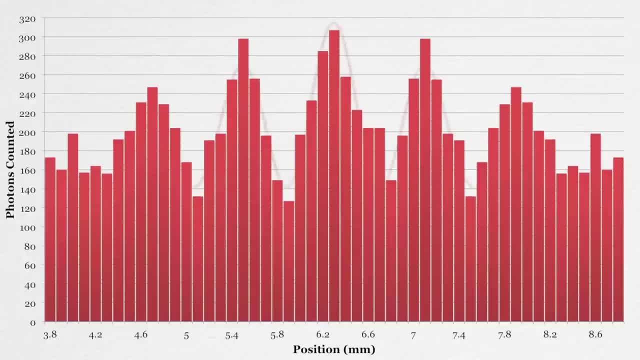 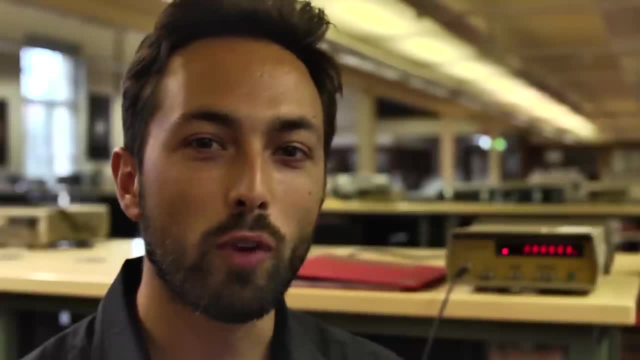 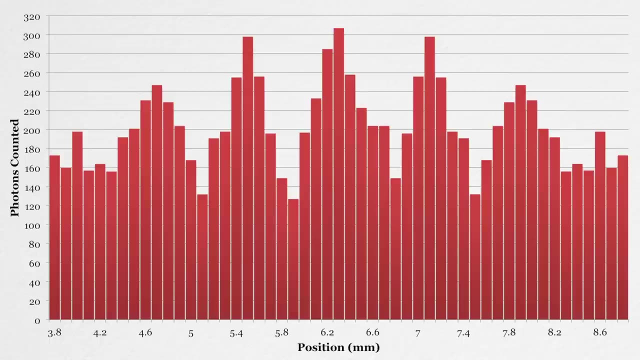 Look at that. You can clearly see the same interference pattern that we got when we were sending tons of photons through. but we're getting it out of single photons, We're counting up individual photons And that pattern is emerging as we aggregate the results over time. 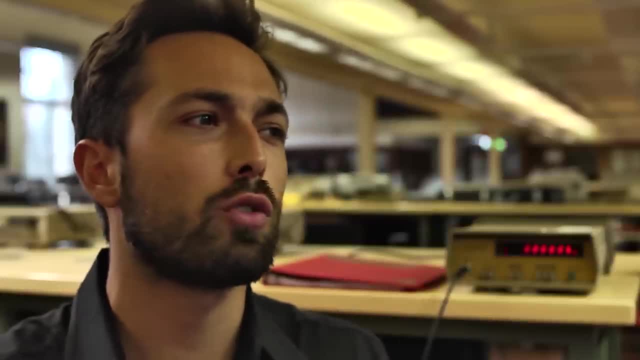 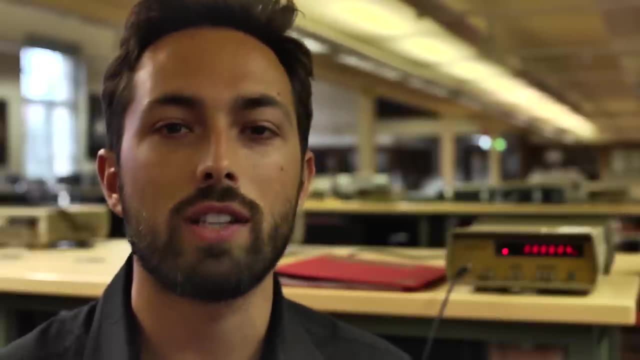 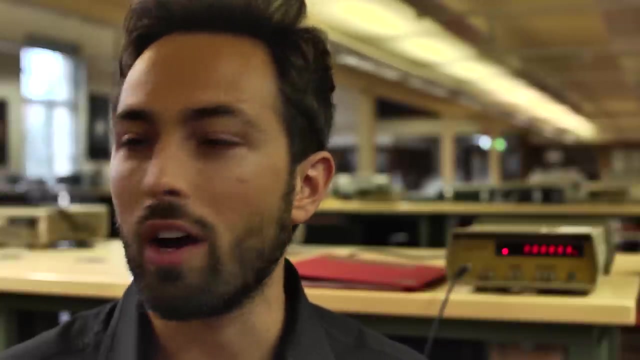 But how could this be happening? How could a single photon pass through both slits? Well, if we try to interpret these results in terms of the objects we experience every day, they don't make any sense. A photon is something different to a macroscopic object. 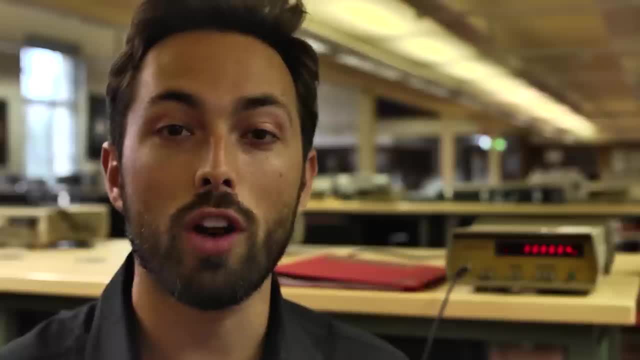 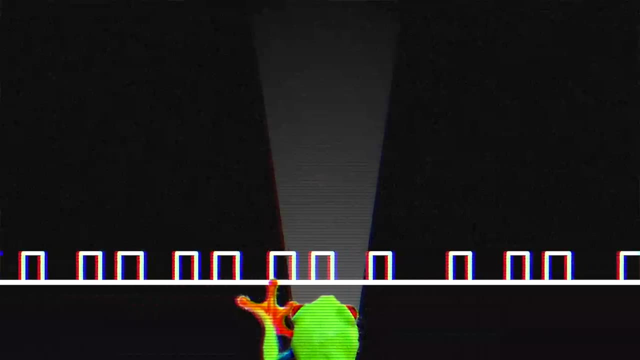 It's not a wave and it's not a particle. It's a quantum mechanical object And sometimes it seems like it has properties of a wave and sometimes it seems like it has properties of a particle, but ultimately it is something totally different to anything we've experienced before. 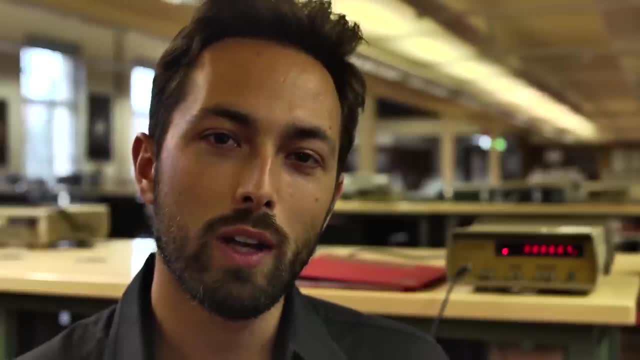 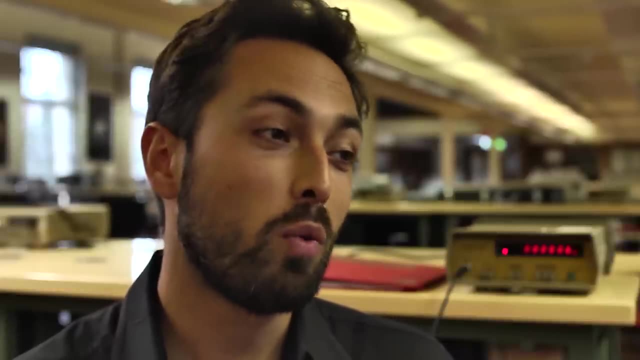 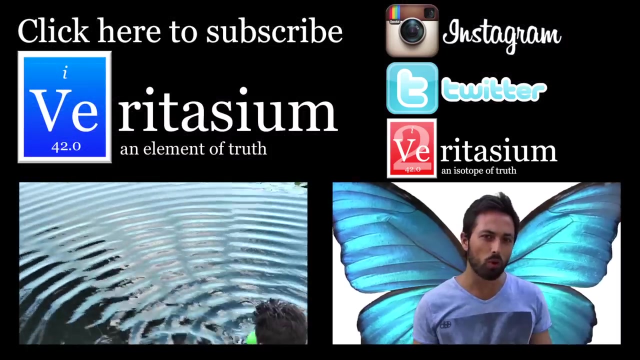 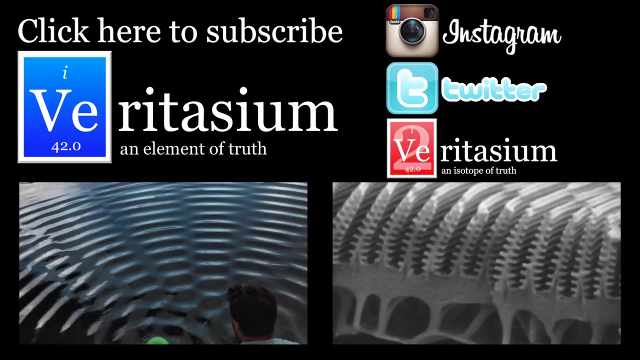 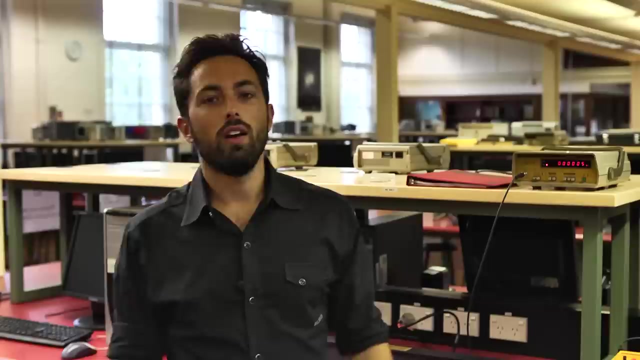 And that's what makes this seem so counterintuitive. So what is light wave or particle? The true answer, I think, is neither, Though, if you want, you could call it a wavicle. At the end of the last video I asked. 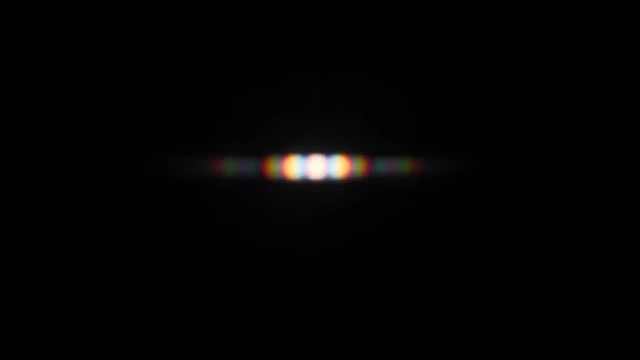 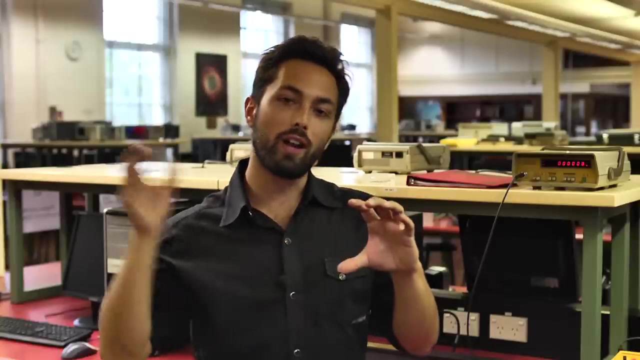 why is it that the interference pattern is made by blobs rather than thin lines of light, as it was in this experiment, And in the comments I saw two common answers. One was that the blobs were images of the Sun and the other answer was that it was due to. 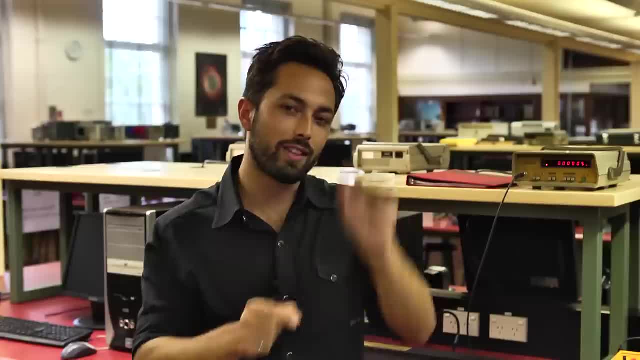 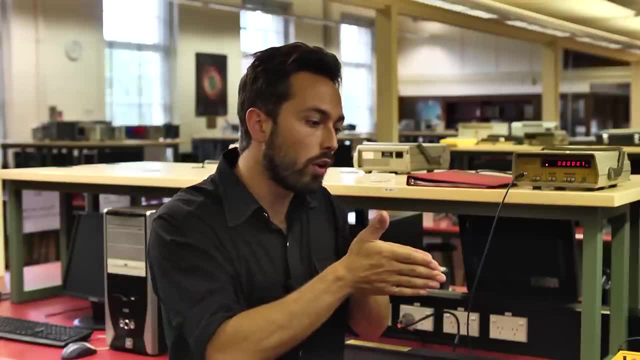 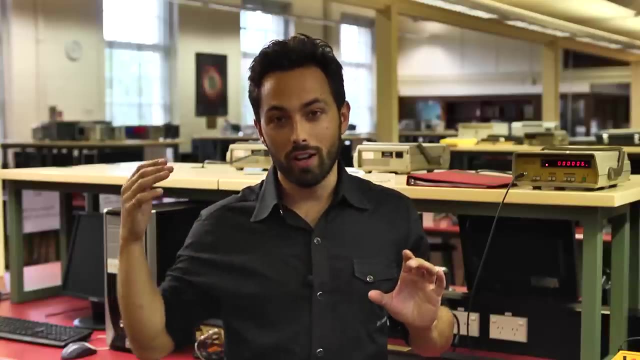 Heisenberg's Uncertainty Principle. Now, those were very thin slits. so it's true Heisenberg's Uncertainty Principle would be involved and that light passing through each slit would spread out. But the reason we actually saw blobs was because they were images of the Sun. 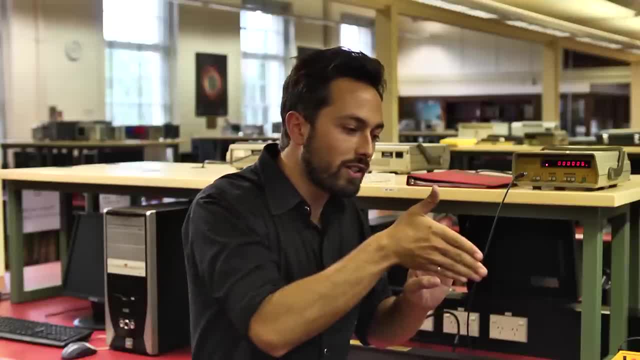 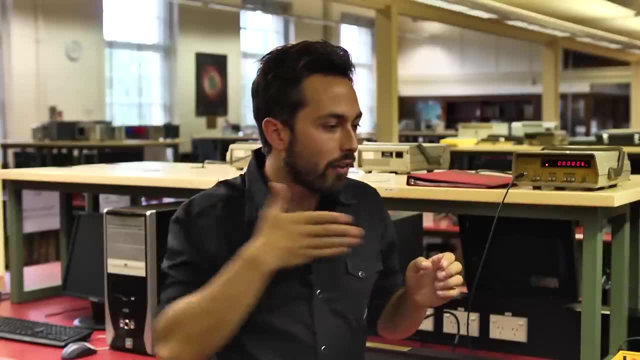 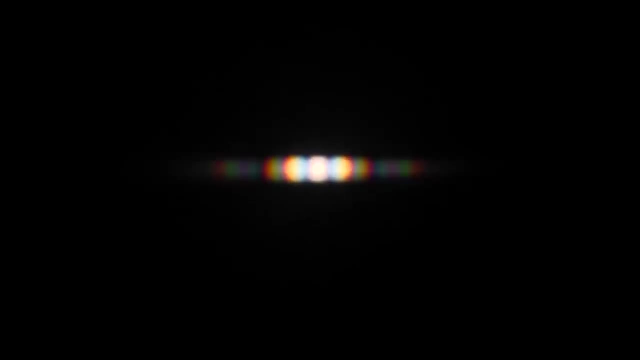 So if the sunlight comes through one slit, it diffracts out and would spread out onto the bottom of the box, And light from the other slit would do exactly the same. And where those two spreads overlap is where we saw the three main blobs. 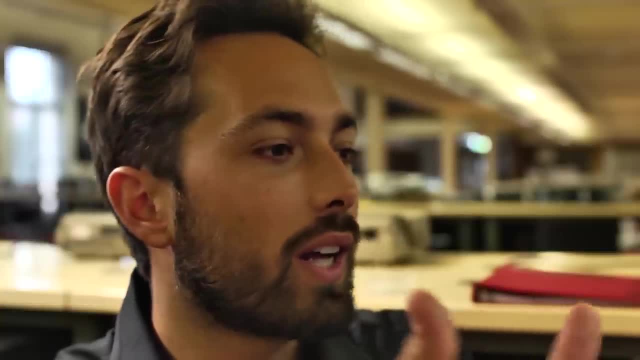 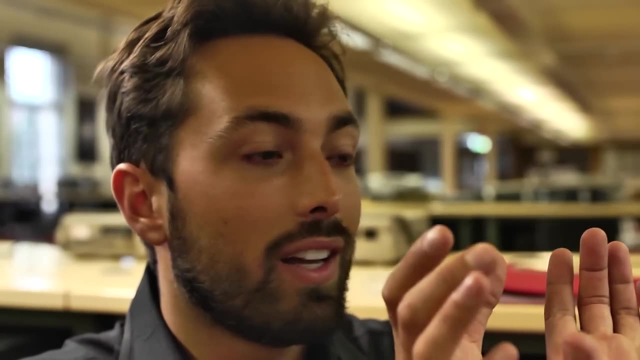 So there's a diffraction maximum created by one slit and another diffraction maximum created by the other slit, and those two overlap, But due to the light being induced, the light being in different phases, it cancels out in certain positions. creating those separate images of the Sun.